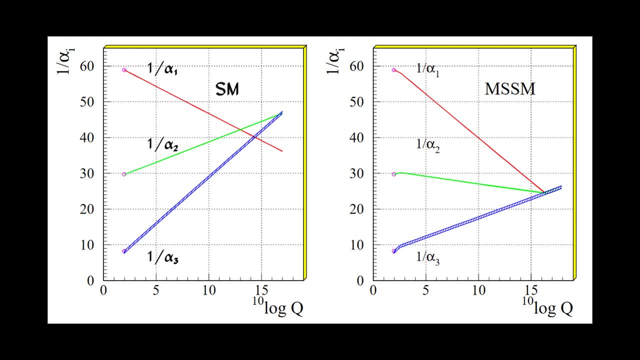 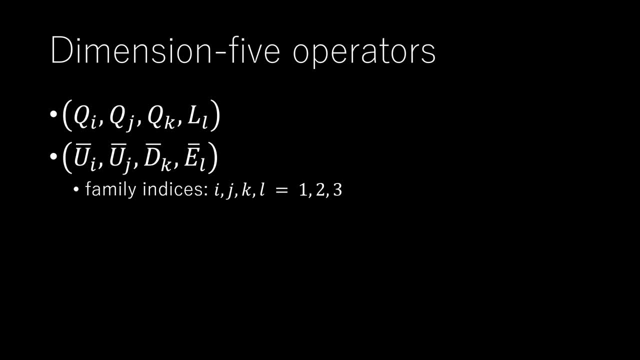 operator. The dimension 5 operators have a dimension-full coupling of order 1 over Mg. The dominant decay modes from dimension 5 operators are p2k plus nu bar. This is due to a simple symmetry argument. The operators qi, qj, qk, ll and u bar i, u, bar j, d, bar k e bar l, where i. j and u bar k are the dominant decay modes from dimension 5 operators: The operators qi, qj, qk, ll and u bar i, u bar j, d bar k, e bar l, where i? j and u bar j are the dominant decay modes. 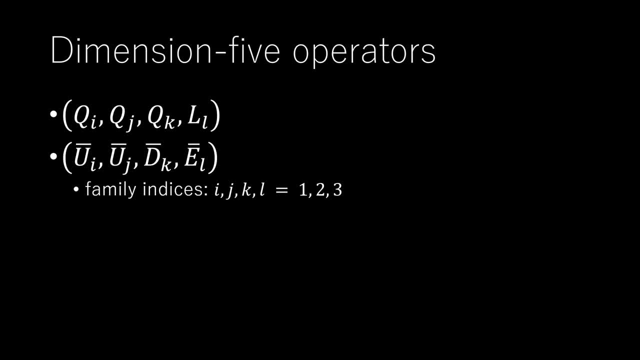 For dates, a, k, l equals one, two, three and family. indices- and color and weak indices are implicit- must be invariant under SU and SU As a result, their color and weak doublet indices must be antisymmeterized. However, since these operators are given by Bosonic superfields, 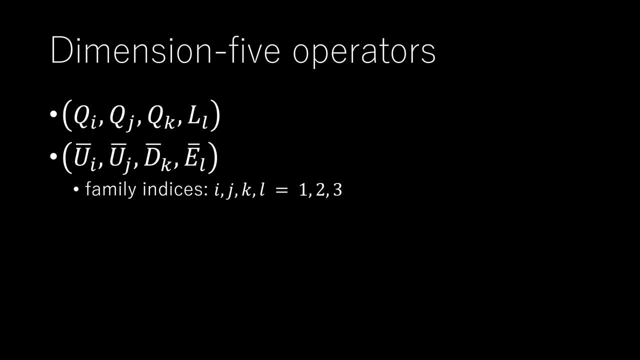 they must be totally symmetric under interchange of all indices. Thus the first operator vanishes, for i equals j equals k, and the second operator vanishes, for i equals j equals k. So the first vanishes, for I equals J. Hence a second or third generation particle must appear. 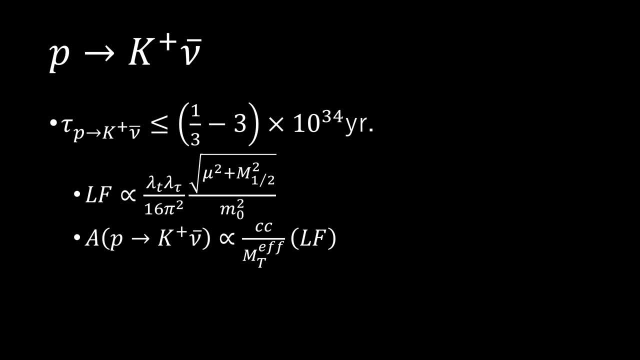 in the final state. The dimension 5 operator contribution to proton decay requires a sparticle loop at the SUSY scale. The loop factor LF is of the form leading to a decay amplitude. A, M½, M0 are the universal gay genome mass. 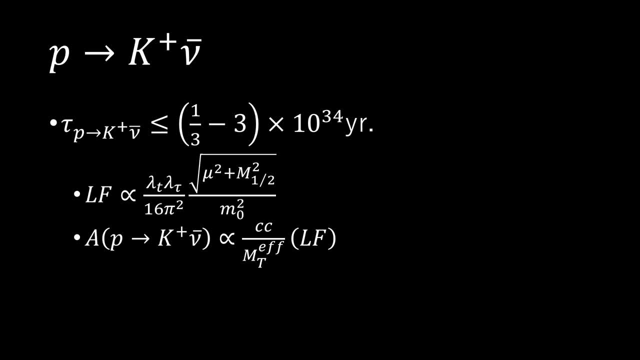 and scalar masses respectively, defined at the gut scale In any predictive SUSY gut. the coefficients C are 3x3 matrices related to Yukawa matrices. Thus these tend to suppress the proton decay amplitude. However, this is typically not sufficient to be consistent. 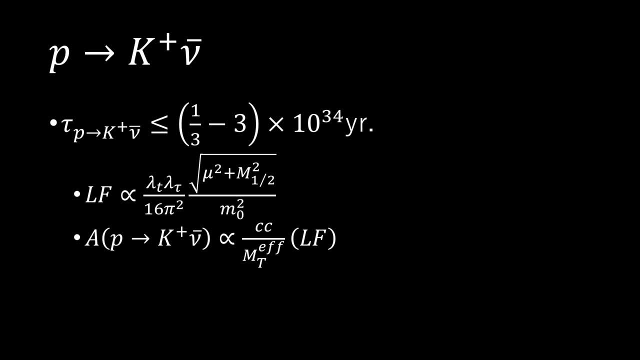 with the experimental bounds on the proton lifetime. Thus it is also necessary to minimize the loop factor. This can be accomplished by taking µ, M½ and M0.. Finally, the effect of Higgs-Culler triplet mass, MTEFF, must be maximized. With these caveats, it is possible to obtain rough. 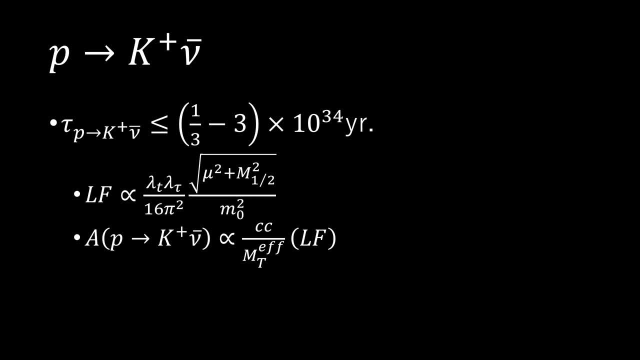 theoretical bounds on the proton lifetime Note: this is close to the super-Kamiokande bound on this decay mode. Future experiments with larger neutrino detectors such as Juno, hyper-Kamiokande and DUNE are planned and will have higher sensitivities. to nucleon decay.